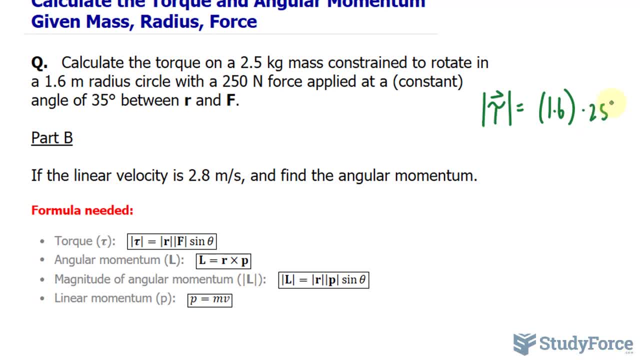 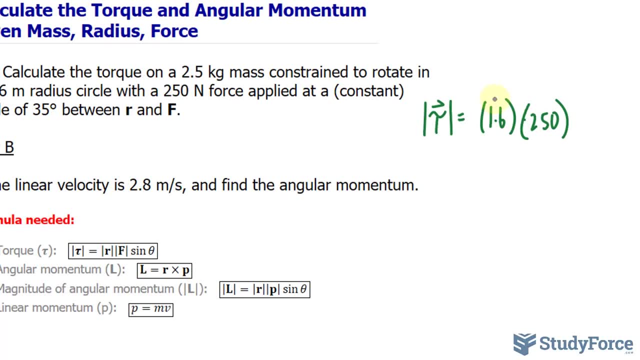 So 1.6 times the force of 250 newtons, And you can always include the units as you're doing this, And let me write down the units so that you don't get confused. So it's 1.6 meters and this one is newtons. 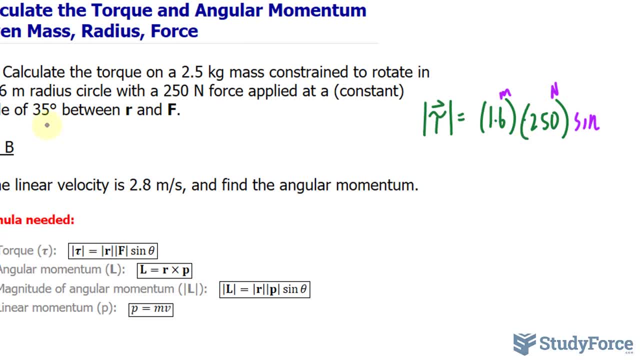 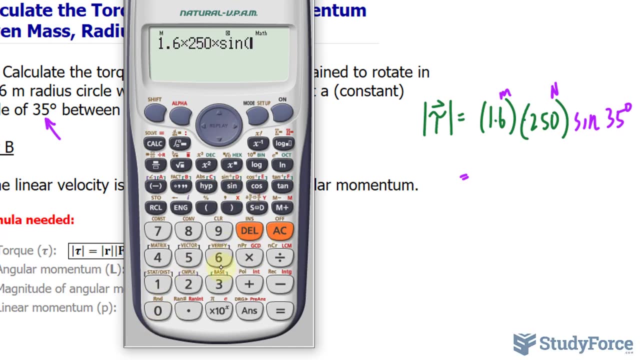 Then we multiply this by sine and the angle is 35 degrees. So make sure that your calculator is in degrees when doing this. So, using our calculator, we have 1.6 times 250, and that gets multiplied to sine 35,. 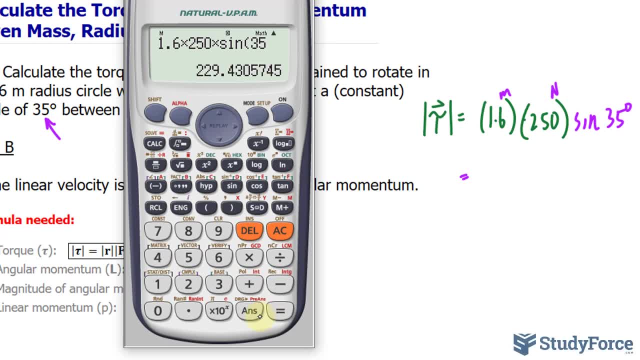 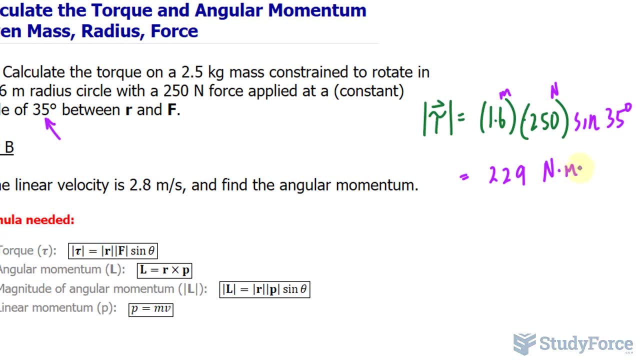 and we end up with a torque that is 229.. I'll just round to the nearest torque value. The units will be newtons times meters. Now I don't want you to confuse these units with joules, because if you break down joules, the unit for energy 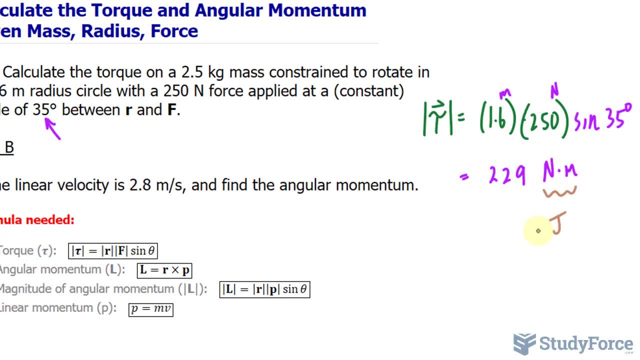 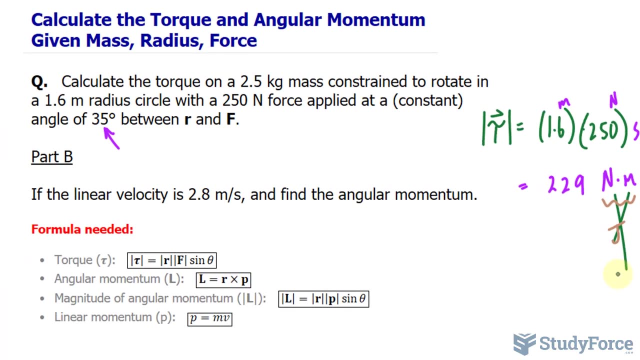 it breaks down into newtons times meters. Except torque isn't a unit of energy, But instead think of it as the rotational version of a force. So this does not equal to a joule, Don't get any ideas. In part B, if the linear velocity is 2.8 meters per second, 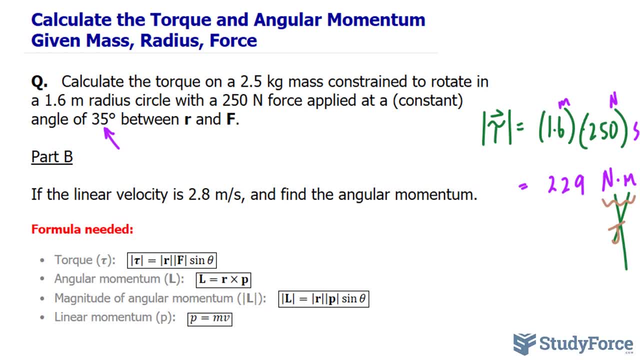 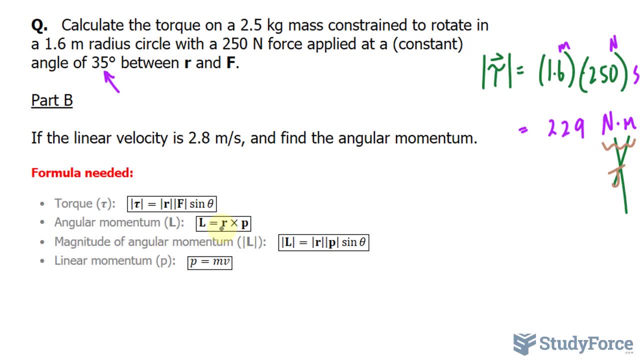 find the angular momentum. Okay, so I've written down here that the angular momentum represented by this vector, L, is equal to the cross product of R times P. That's said differently: R cross P And P represents the linear momentum. We've worked with this in the past. linear momentum. 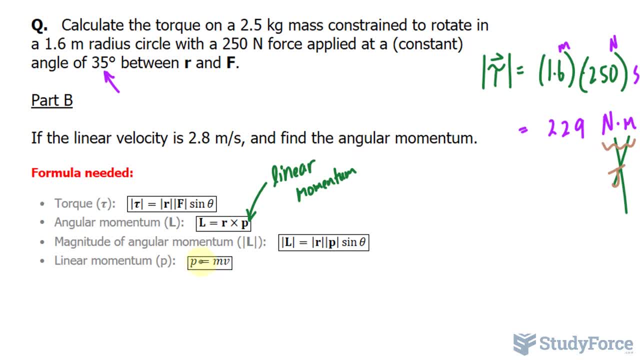 And the formula for linear momentum shown right here is mass times velocity. Now, it's not specified here, but we're not looking for the vector components of the angular momentum. Instead, we're looking for its magnitude, And the magnitude can be found using this formula. 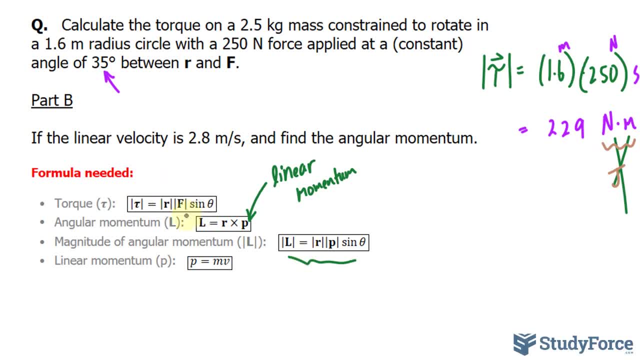 Notice that it's very similar to the formula we used up here, where we multiply the magnitude of the radius times, the magnitude of the linear momentum, and that gets multiplied to the angular which that's occurring. So what I will do is take this value of 2.8.